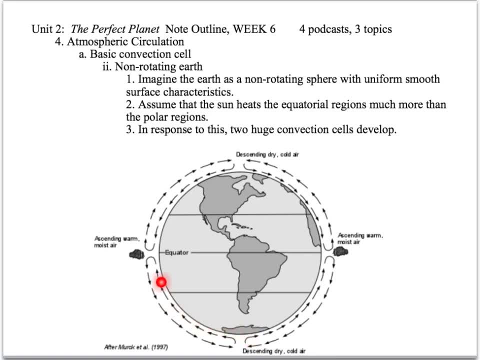 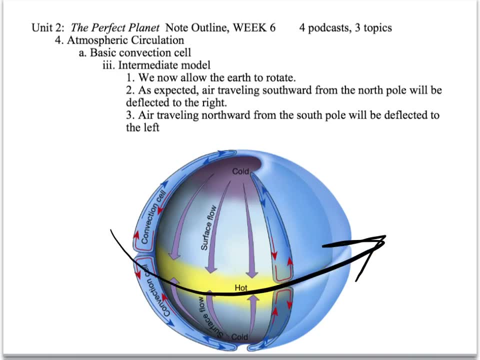 moving hot air north and then cold air, or south and then cold air back to the equator. Alright, so now let's rotate the Earth and see what happens. We'll rotate the Earth in this direction, which is appropriate, and so what's going to happen? 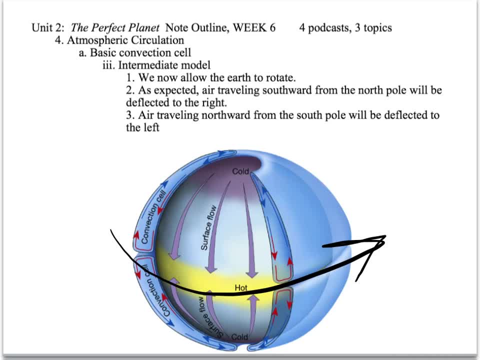 to the atmospheric convection, We're going to notice that it's going to look like air traveling southward from the North Pole will deflect to the right and air traveling northward from the South Pole will deflect to the left. This might be easiest to understand if you think about it from the point of view of. 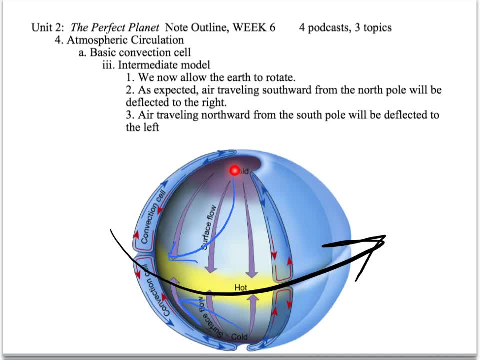 an airplane flying from the North Pole south to a city near the equator. Imagine an Earth that rotates, which it does, and imagine the airplane leaves and flies directly south. Well, instead of landing. if it flies directly south instead of landing? 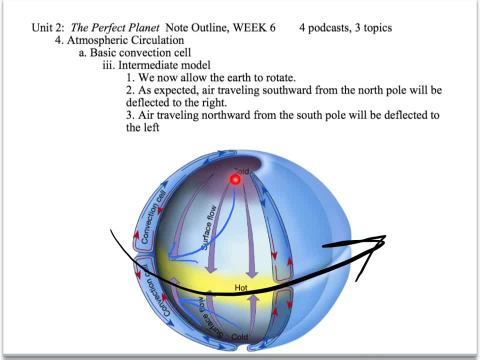 at a point on the equator directly south of it. it's actually flying south, but as it's flying south, the Earth is rotating, so it's going to deflect to a city that is actually to the west of where it had intended, unless it actually, as it flies as the airplane. 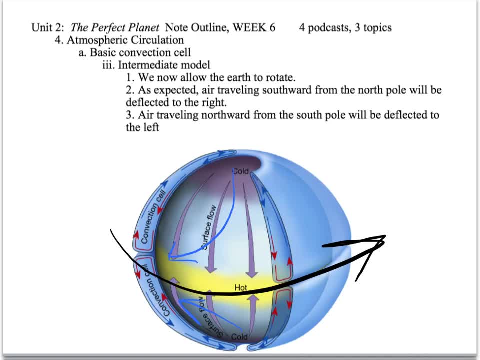 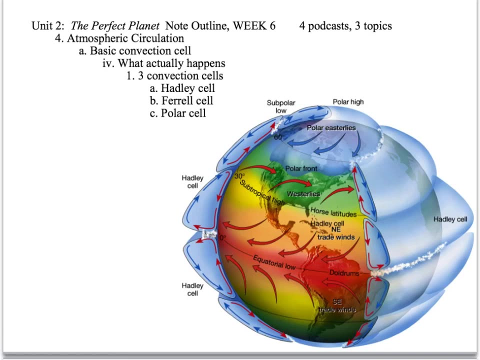 flies, unless it actually angles the plane so that it can fly. It can actually steer it to try to fly where it's supposed to get to as the Earth rotates away from it. Alright, so as if that wasn't complicated enough, it gets one step more complicated. 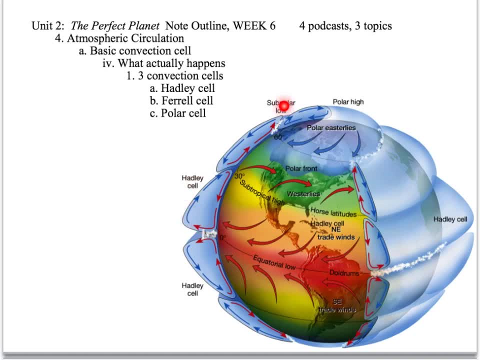 Interestingly enough, we don't see one gigantic convection cell in the North and one gigantic convection cell in the South. We actually see three identical convection cells in the North and South, So we have a Hadley cell. So air that rises at the equator is going. 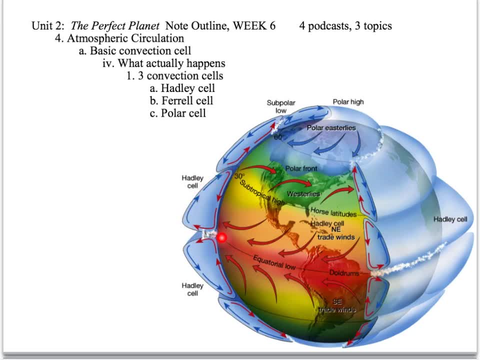 to deflect off. You can see, from the Jeez 수 to the north n the northern hemisphere and to the south in the southern hemisphere, And it's only going to make it as far as thirty degrees north or south. and that air which rose as warm, humid air and then precipitated, 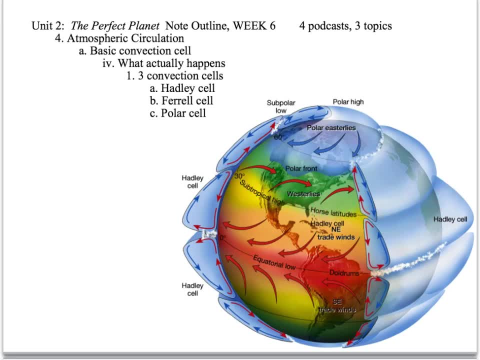 out is going to fall as dry warm air, And so that's where a lot of the Earth's deserts are, at those thirty degree north and south latitudes, because the warm air is also dry convection. The ferrule cell is between 30 and 60 degrees north and south and the polar 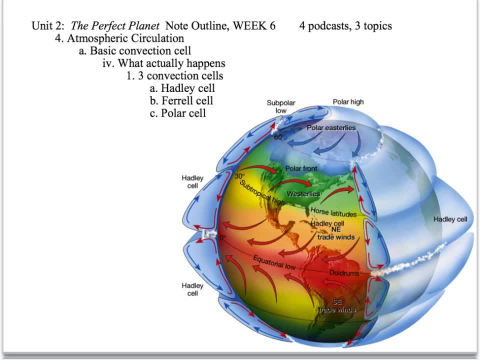 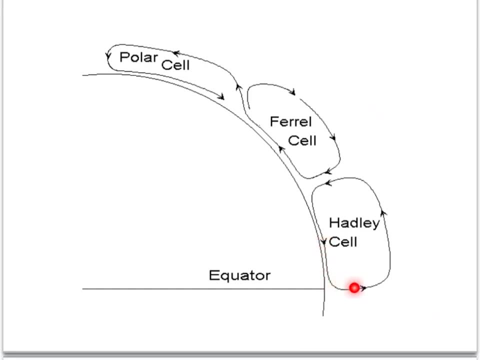 cell is at either the north pole and the south pole. So here's the same thing, just a different way to look at it: Hadley cell, convection, ferrule cell and then polar cell. And the same thing again. just interesting to check out the different pictures, different ways. 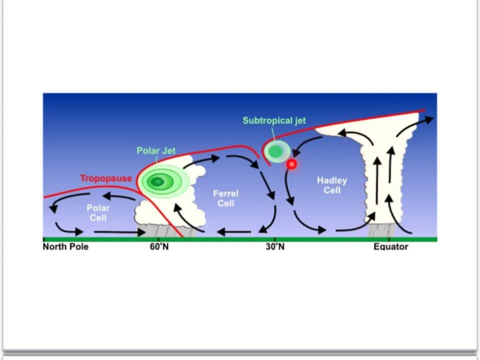 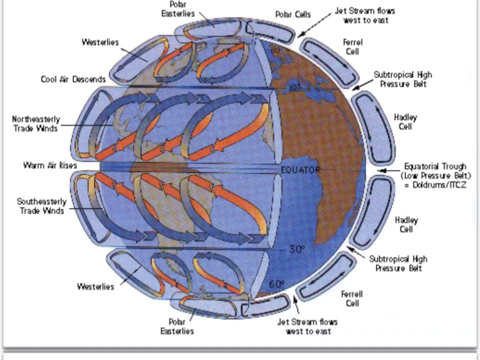 to visualize this, Here's the equator right here: Hadley cell, ferrule cell, and then the polar cell. And again here's the equator: Hadley cell, Hadley cell, ferrule cell, ferrule cell, and then the polar cell, and then the polar cell At the point where they had the 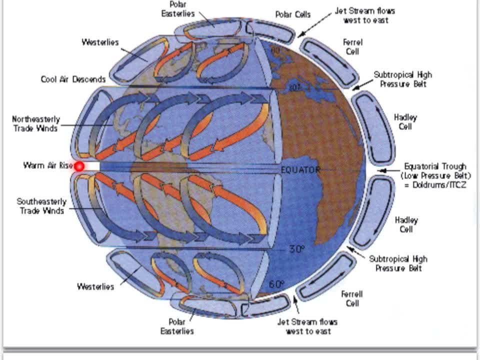 Hadley cell comes across the other Hadley cell, so the northern Hadley cell comes across and meets the southern Hadley cell. That's called the doldrums or the ITCZ, which is the intertropical convergent zone, And that's where we see warm air rising at this point. 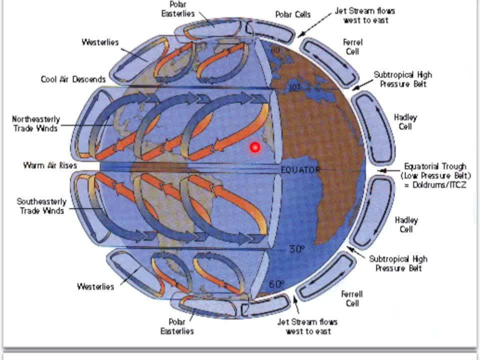 It is warm, it is humid and you're going to get a lot of rainforests in this region, right at the equator, obviously, Where the Hadley cell, and we'll just look in the northern hemisphere, where the Hadley cell comes across and meets the ferrule cell, you have air and 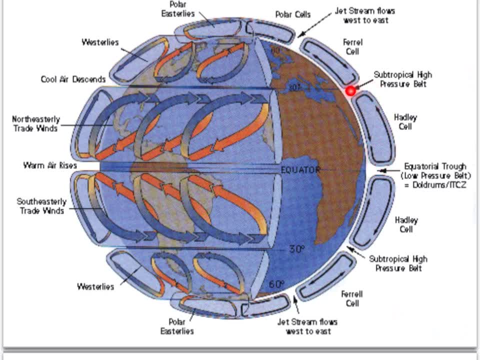 air that is descending, And the air is warm because it was warmed at the equator, but it's also dry. It's already rained and precipitated, And so this is where the world's deserts in general are located, at 30 degrees north or south. Cool air is descending here and warm. 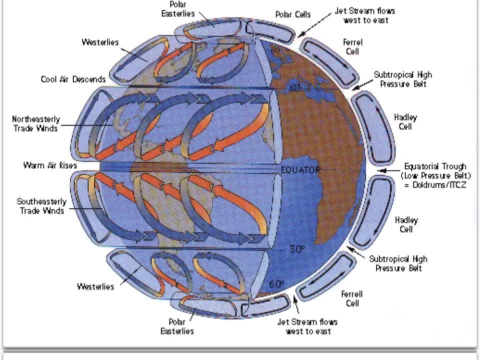 air is descending here. It's cool if it came from the ferrule cell and it's warmer if it came from the Hadley cell And where the ferrule cell meets the polar cell that you get a jet stream there. Jet stream flows west to east. 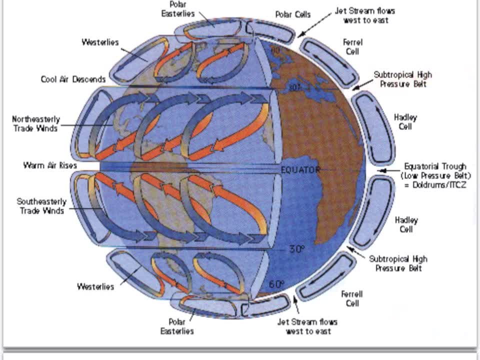 We'll talk briefly about high pressure belts. High pressure is when you get descending air. So you get descending air here as the air is coming down and crashing down on the earth. That is high pressure. Low pressure is caused by air that's rising. The air is leaving the 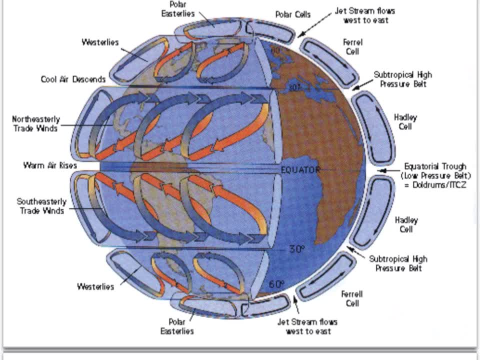 earth here, so that the pressure is low. And again you're looking at why. what's the deal with these circles here? Well, it's again because of that- the rotating earth, The air is deflecting and then it's returning, and then it's deflecting because of the 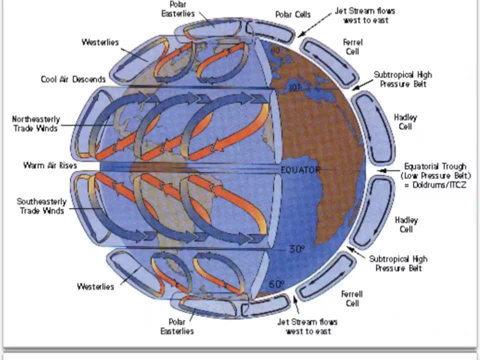 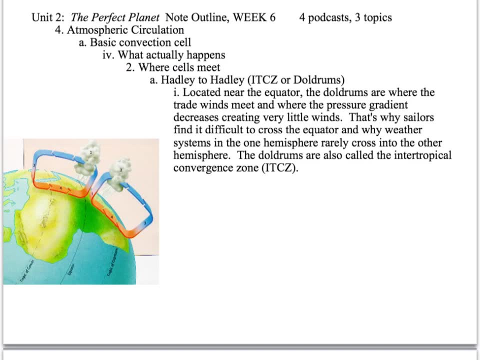 fact that the earth is rotating. It's the Coriolis effect. Now, hopefully, that video on the last slide worked for you. I'm still learning how to do all this stuff, So feel free to pause this slide if you need to write this down. 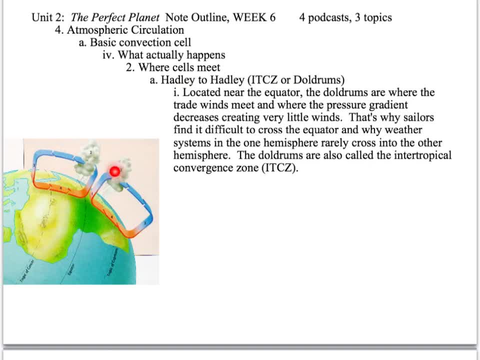 but Hadley to Hadley cell again. I've already said this, but that's at the equator right And that's called the doldrums. Sailors find it hard to cross here because air is moving up instead of across. That makes sense. Also called the intratropical convergence zone. 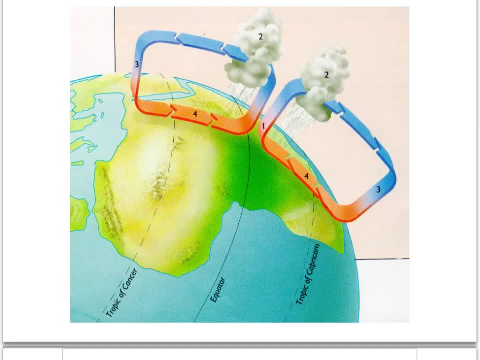 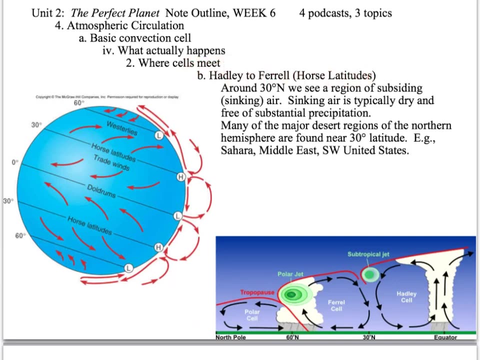 So Warm air, rising Humid. Yeah, There's just a close-up. Yep, Feel free to pause this one if you need to too. Hadley to Farrell cell called the horse latitudes. Again, that's 30 degrees north and south, Sinking air, high pressure system, Major deserts around this. 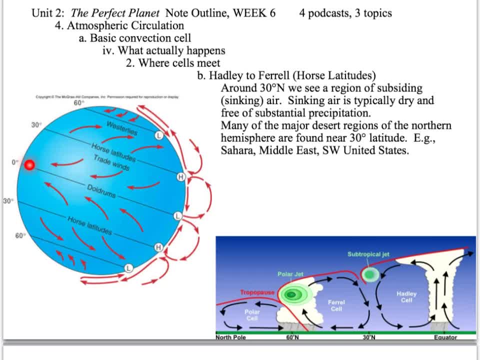 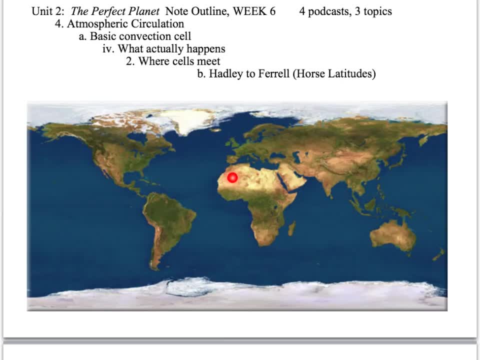 area because you know it already rained. The precipitation from the warm, humid air has already left, Again called the horse latitudes And you can see Earth deserts there, right Here's the equator, Here's the intratropical convergence zone. 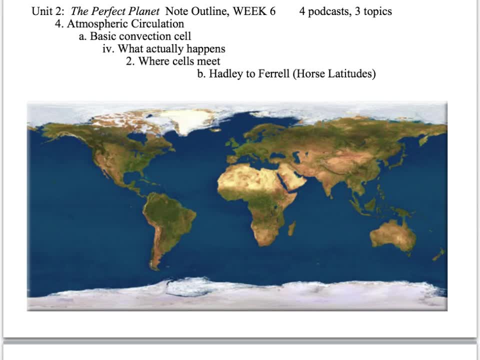 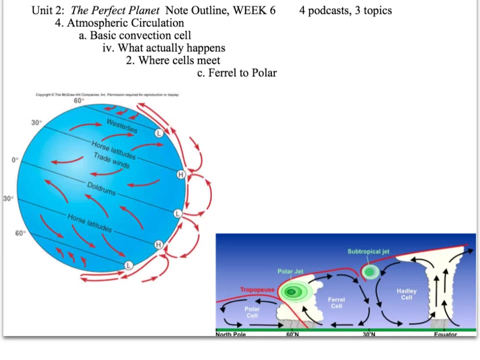 Warm air, rising Humid. So the warm air rises at the equator and it rains, and then the warm air, which is now dry, falls and there is your deserts, All right, And finally, at 60 degrees latitude north and south, you do get rising air again, as the Farrell cell. 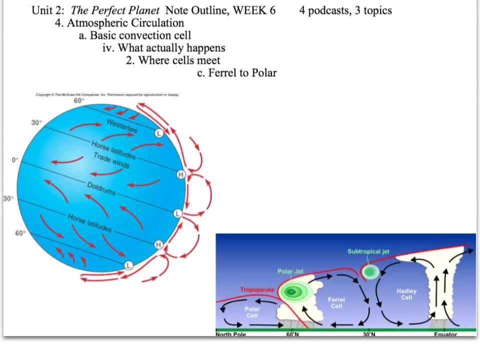 hits the polar cell. There's a polar jet stream there, Subtropical jet stream there. I forgot to mention All right, And yeah, There's that, All right. Hopefully this podcast made sense and I'm going to call it good And have a good one.